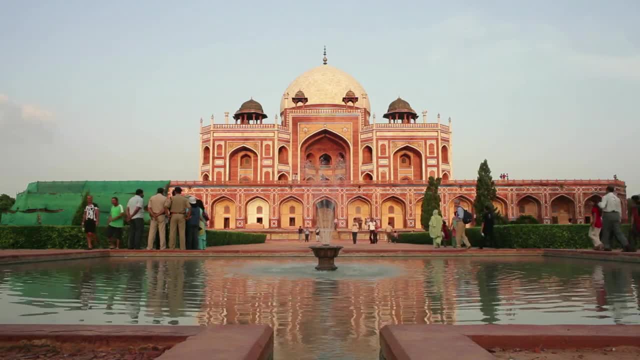 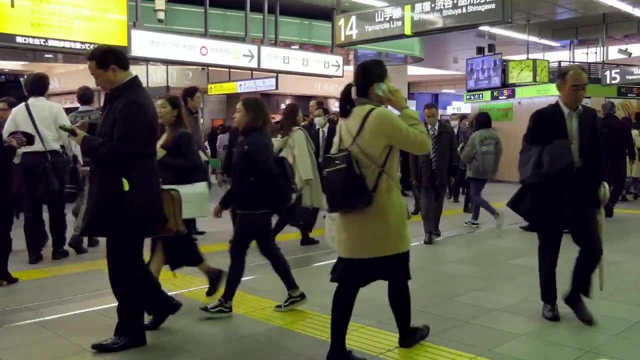 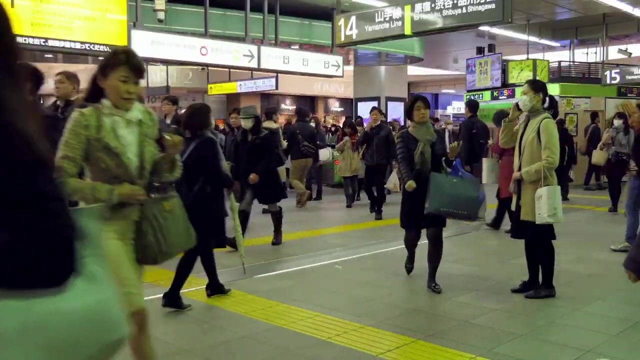 which means the population is increasing, But very slowly when compared to what happened in the past two centuries. The population of many countries such as China, Brazil, Japan and Germany will be stagnant or even decreasing in 2050.. The region of the world that will grow the most will be the African continent In Africa. 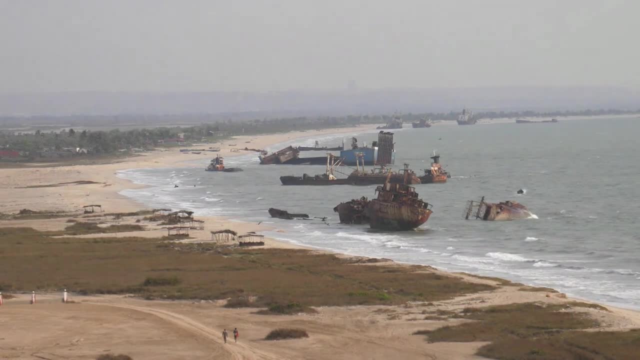 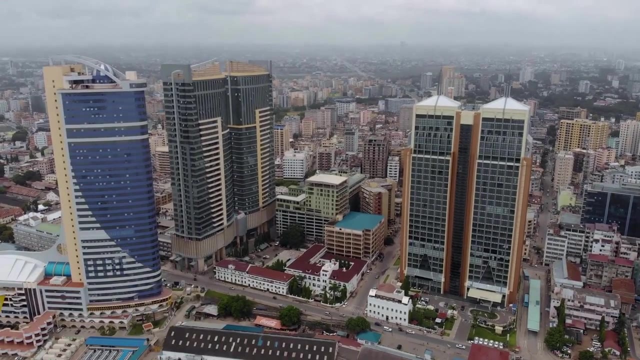 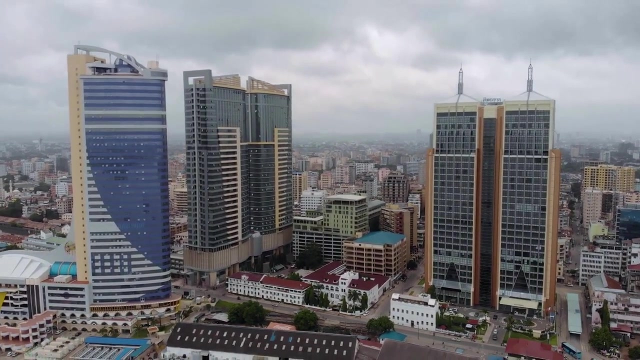 the fertility rate is 4.7 children per woman, which is almost double the world rate. Despite political instability in many countries, Africa is expected to increase its GDP volume considerably, and the population growth may represent a danger to the environment. Anyway, it is not possible to predict exactly what will happen to the environment in the next decade. 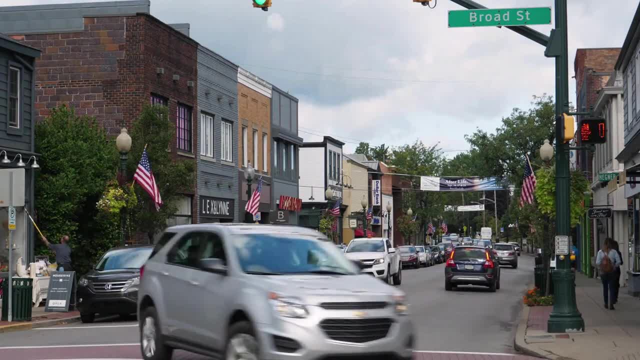 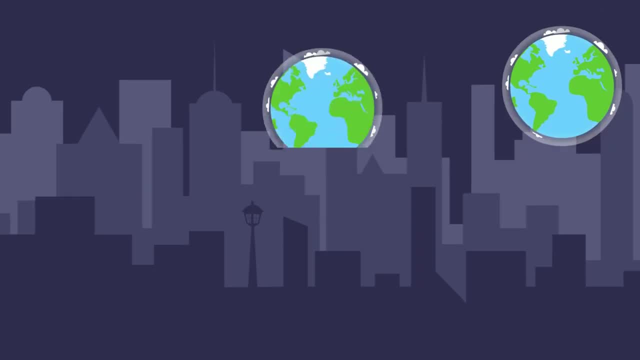 But with our lifestyle and consumption today it is not possible to imagine that all countries on the planet can achieve the lifestyle of developed countries. For example, if everyone in the world consumed as an average American, we would need 5 Earth planets to sustain us. Of course it does. 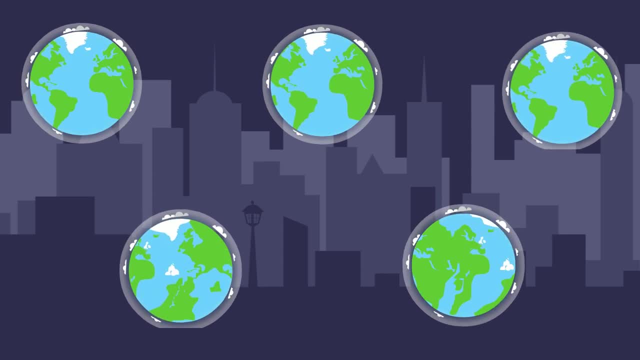 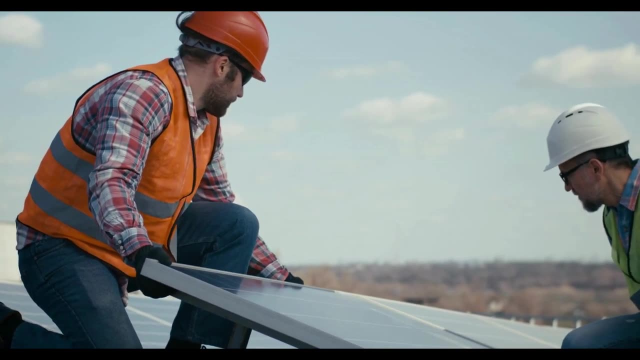 not lead us to the conclusion that we must prevent poor countries from improving their quality of life. It is much more fair and efficient to invest in technologies that reduce the waste produced by humans and that also make clean energy sources cheaper, which will reduce the burning of fuels. 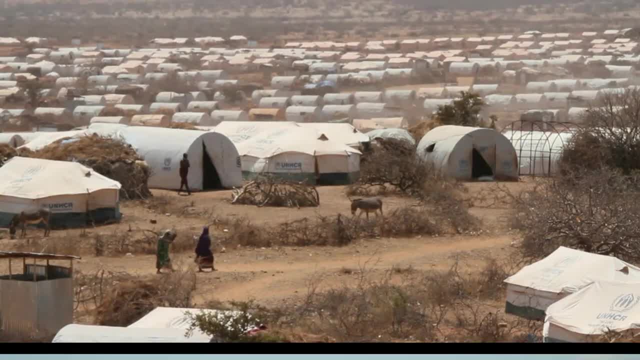 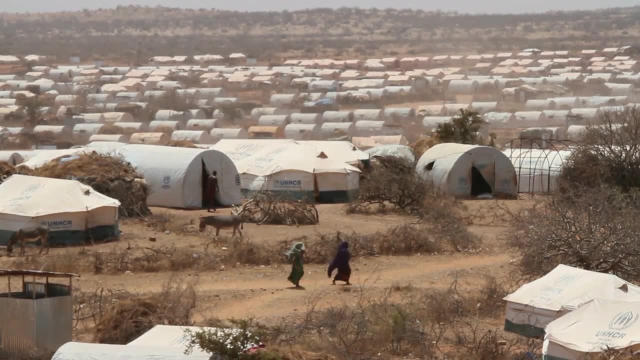 The UN says that the best ways to decrease the fertility rate are birth control with preventive public policies such as the distribution of condoms and contraceptives. Furthermore, to educate the population, especially women. When a woman is in the labor market, the probability 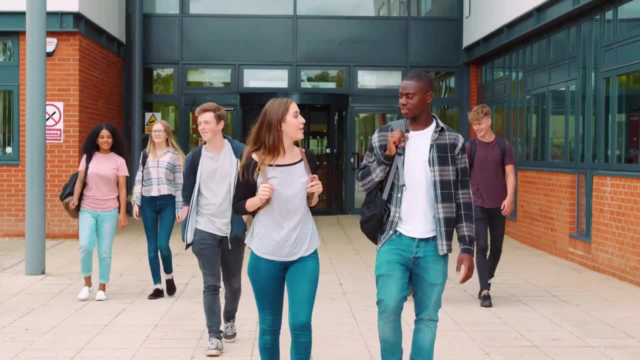 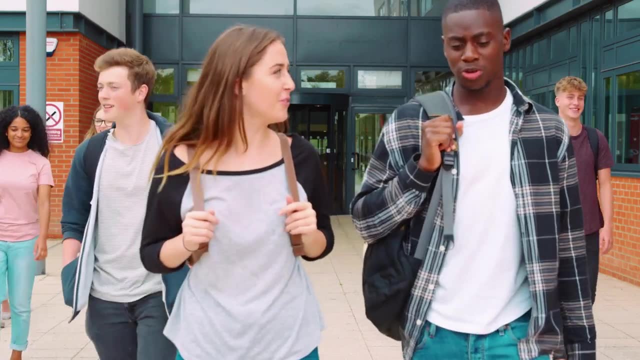 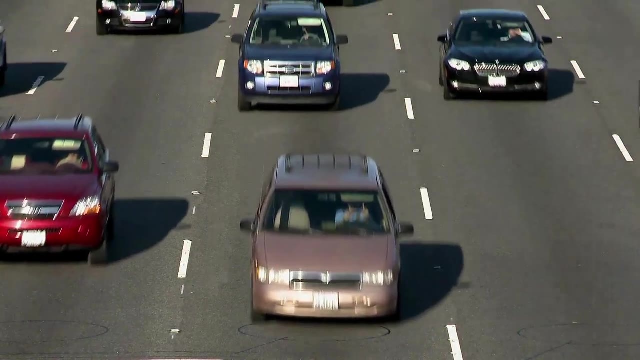 her having many children are considerably reduced. in addition, educating and raising awareness among the population reduces the number of children and creates better living standards for the whole family. to reduce the human impact on the environment, the decrease in excessive consumption is essential. only a few people care about the environmental consequences of their behaviors. 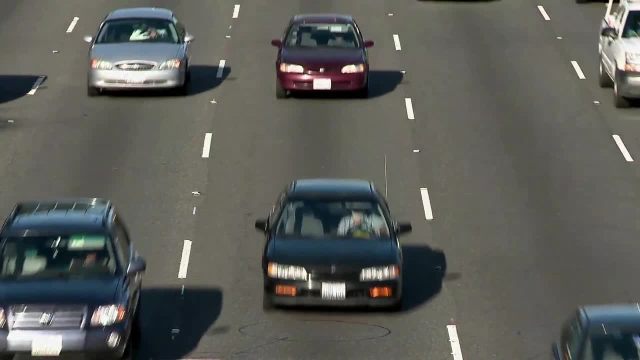 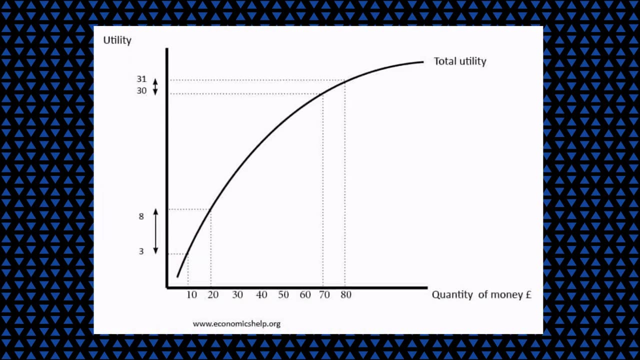 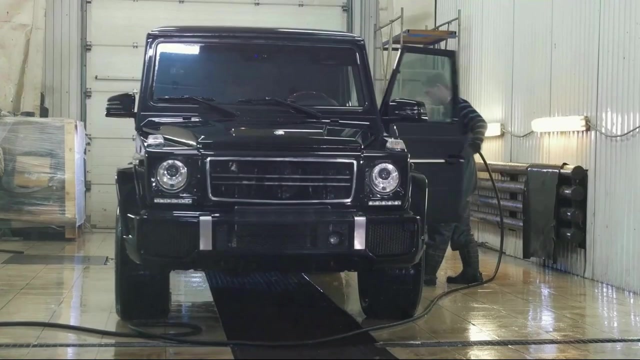 almost no one cares about the environmental impact of their cars or the process of producing their clothes. most of them only make a correlation between the satisfaction generated by that product and the available budget. the concern with the environmental impact is almost zero. not many people will withdraw from buying a pickup truck or an suv because of its environmental impact.